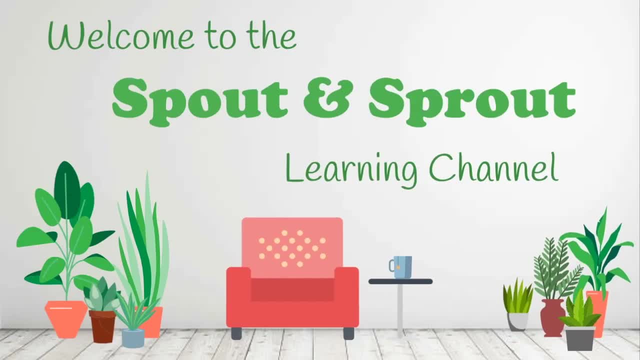 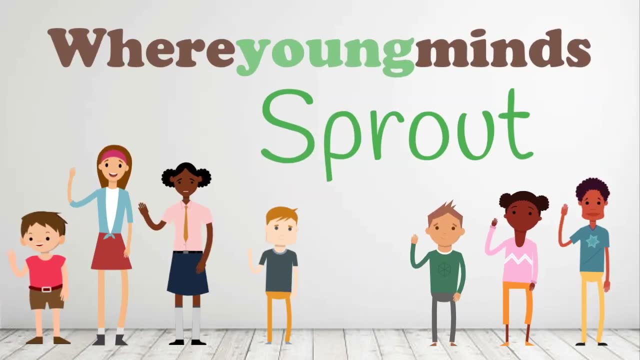 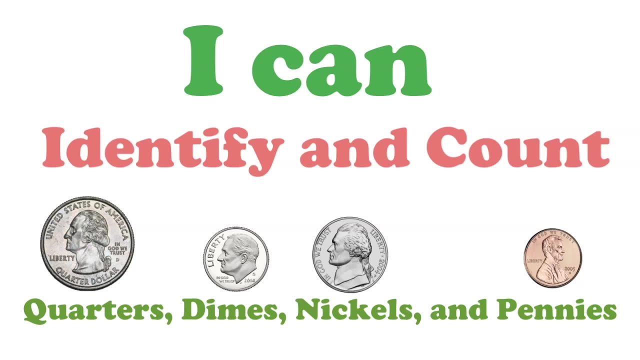 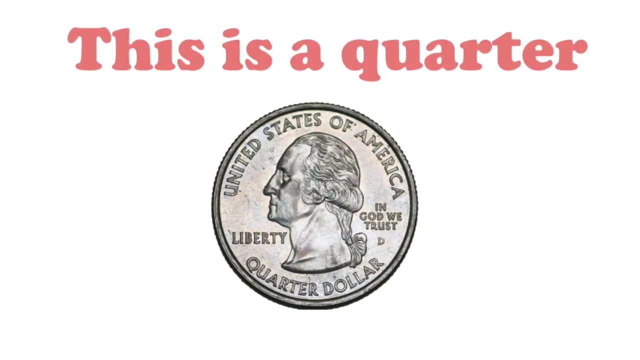 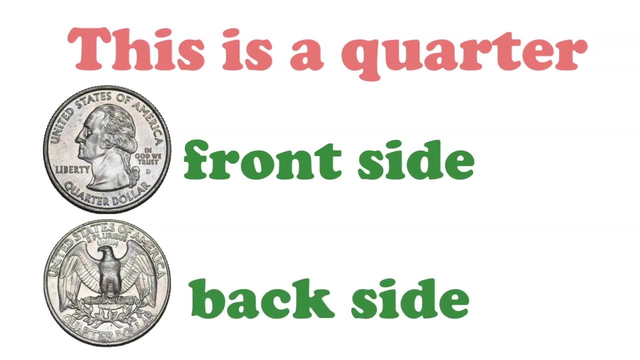 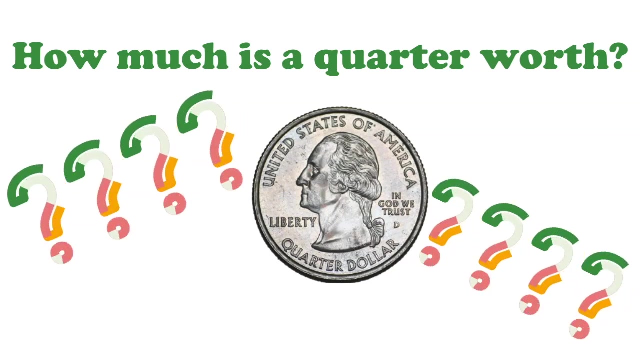 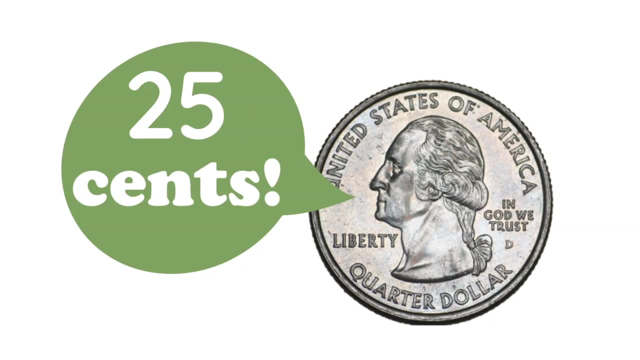 I can Identify and count Quarters: dimes, nickels and pennies. This is a quarter, This is the front side and this is the back side. How much is a quarter worth, Do you know? Yes, it is worth 25 cents. 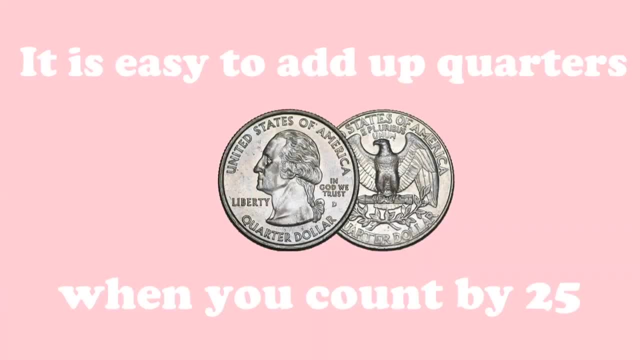 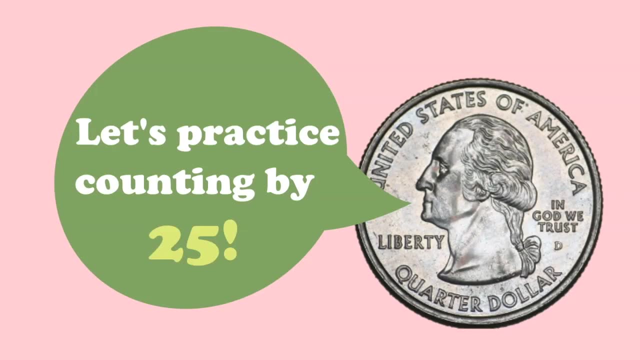 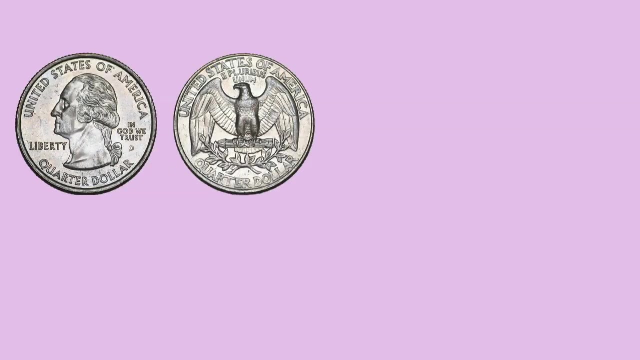 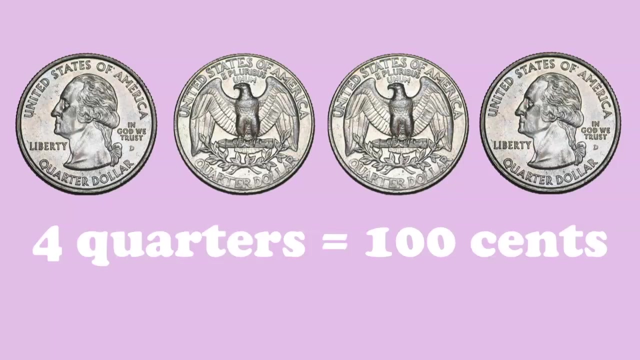 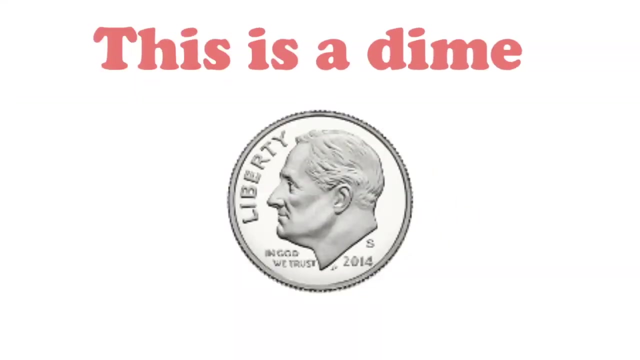 It is easy to add up quarters when you count by 25.. Let's practice counting by 25.. 25,, 50,, 75, 100.. Four quarters equals 100 cents. 100 cents equals one dollar. This is a dime. 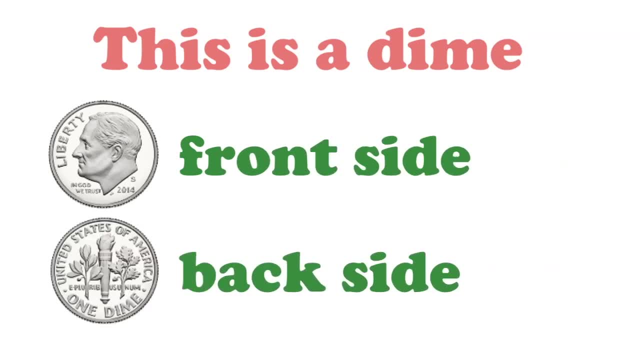 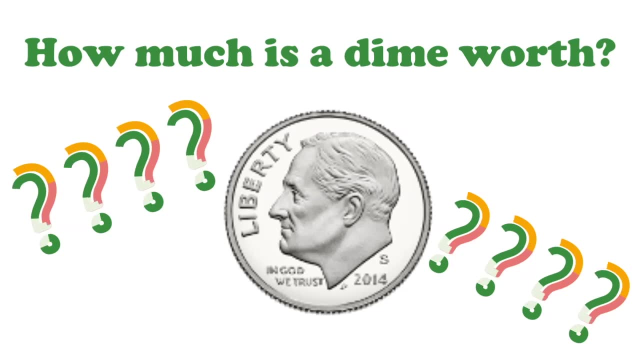 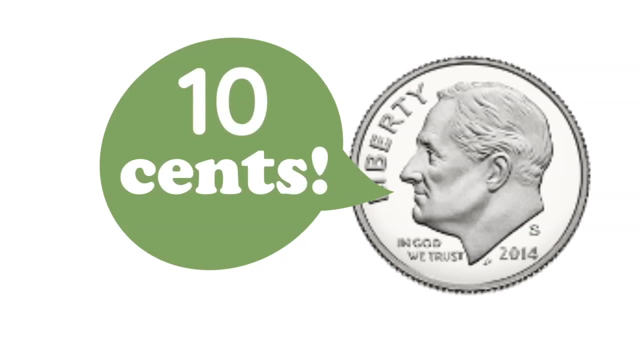 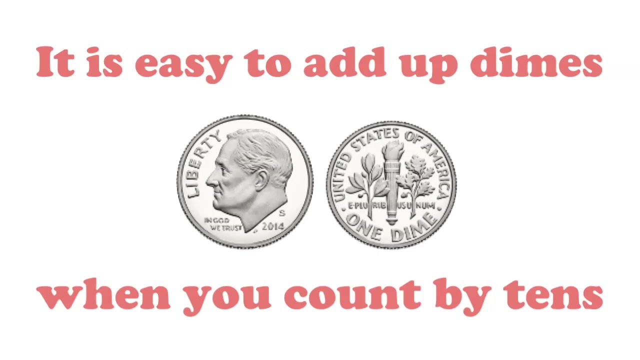 This is the front side and this is the back side. How much is a dime worth, Do you know? Yes, it is worth 10 cents. It is easy to add up dimes when you count by 25.. This is the back side and this is the front side. 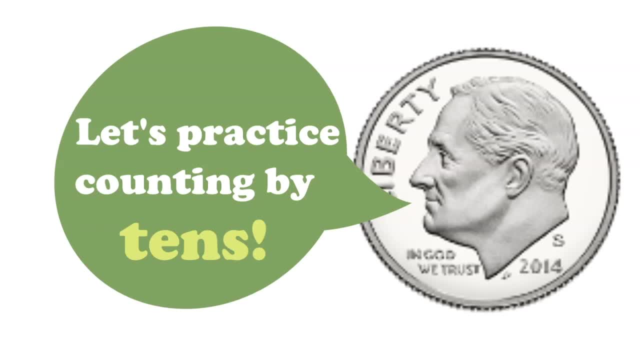 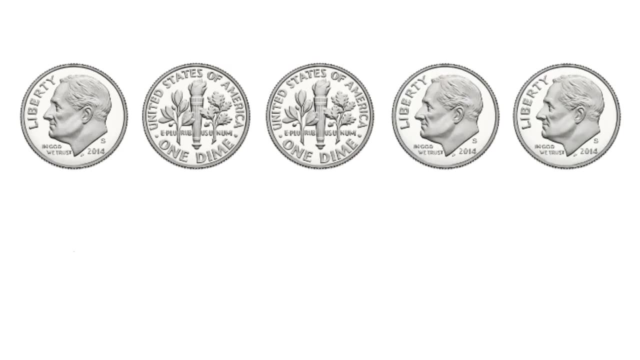 This is the front side and this is the back side. Just add up each row of quarters: 20,, 25,, 60,, 70,, 80,, 90,, 100.. How much is a quarter worth 10.. 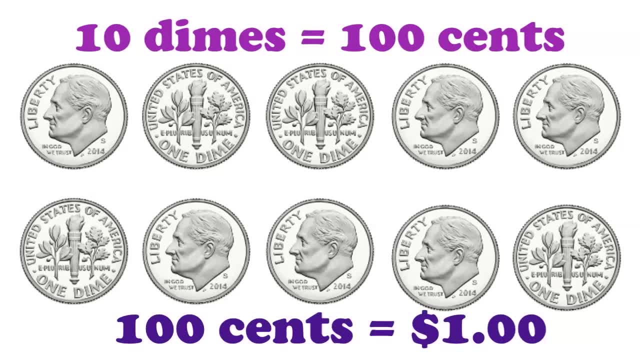 Let's practice counting by tens: 10,, 20,, 30,, 40,, 50,, 60,, 70,, 80,, 90, 100.. How much is a dime? How about a ten? It's a bonus. 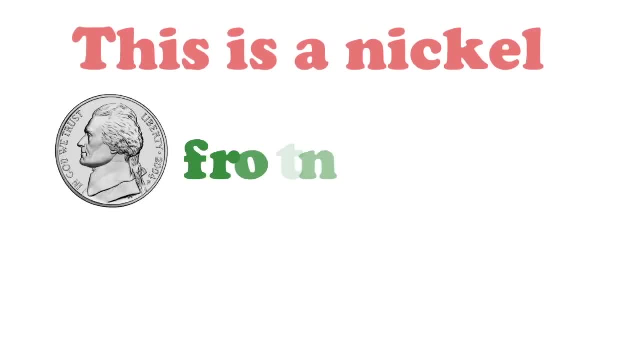 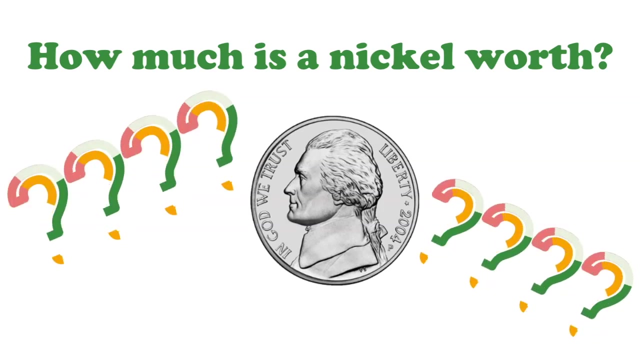 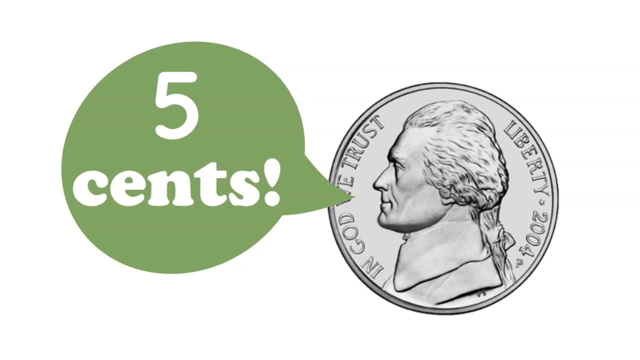 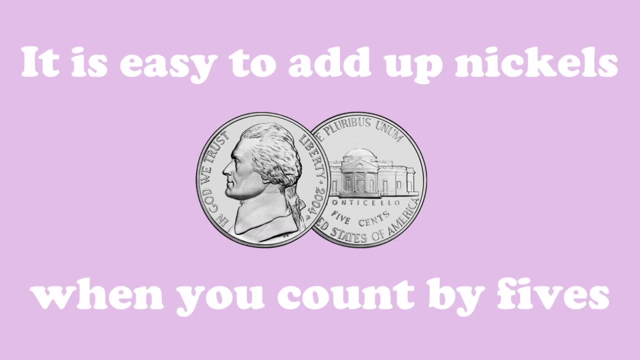 electricsenet nickel. This is the front side and this is the back side. How much is a nickel worth, Do you know? Yes, it is worth 5 cents. It is easy to add up nickels when you count by fives. 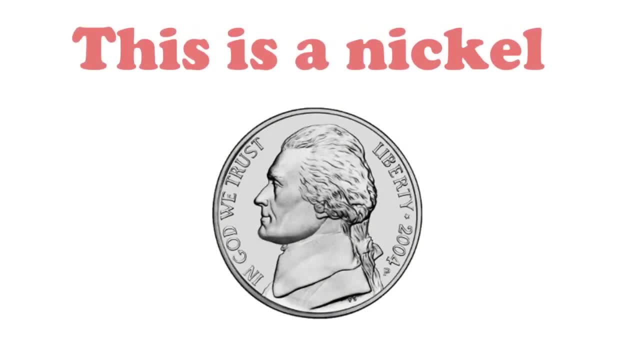 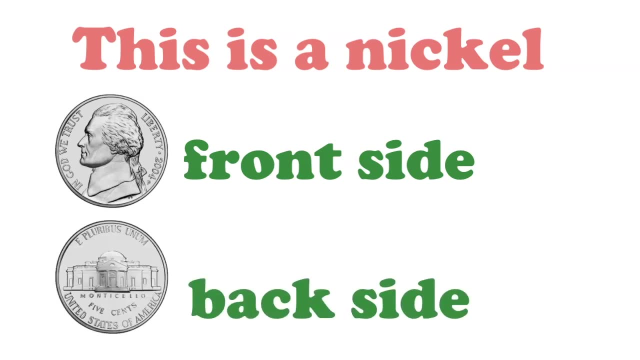 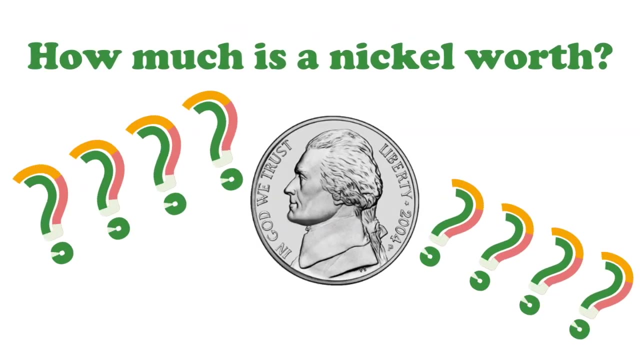 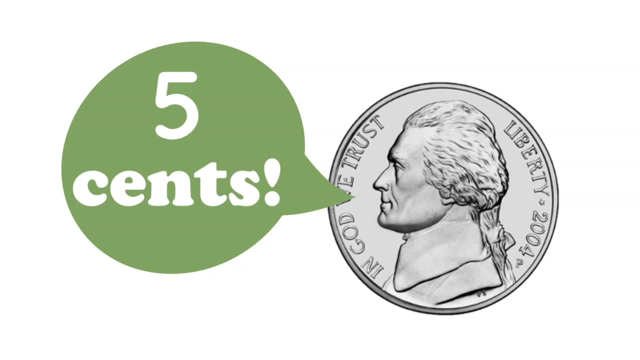 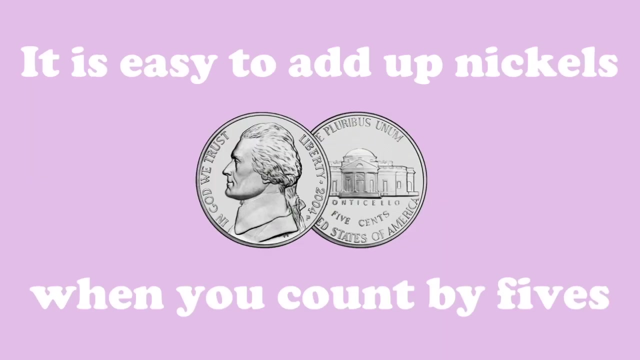 $1.. This is a nickel. This is the front side and this is the back side. How much is a nickel worth, Do you know? Yes, it is worth 5 cents. It is easy to add up nickels when you count by fives. 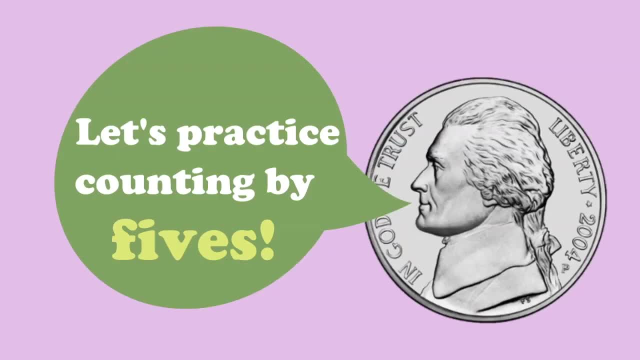 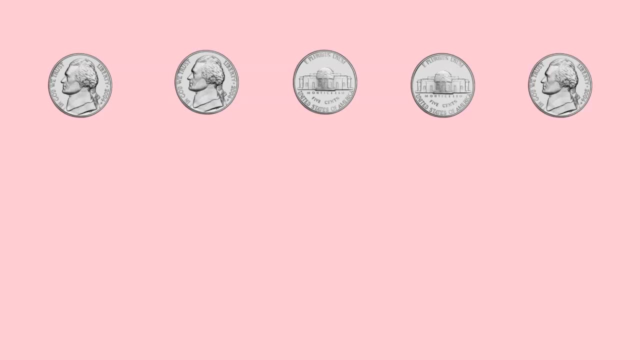 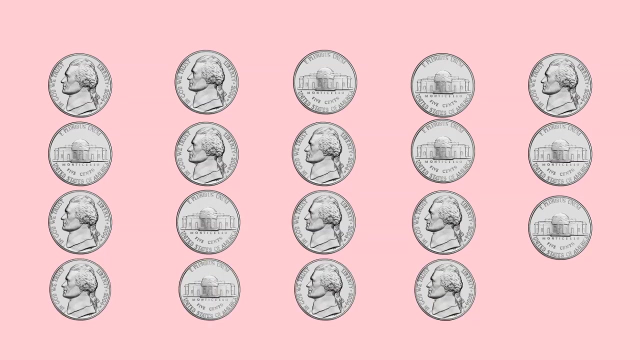 Let's practice counting by fives: 5, 10,, 15,, 20,, 25,, 30,, 35,, 40,, 45,, 50,, 55,, 60,, 65, 70,, 75, 80,, 85,, 90,, 90, 90, 90, 90, 90,. 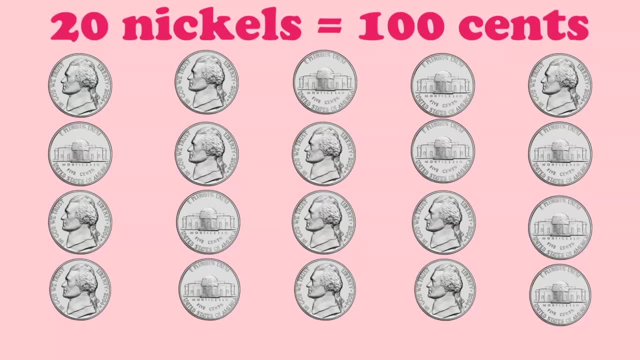 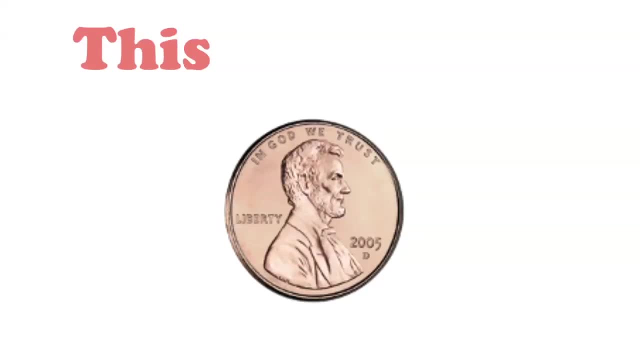 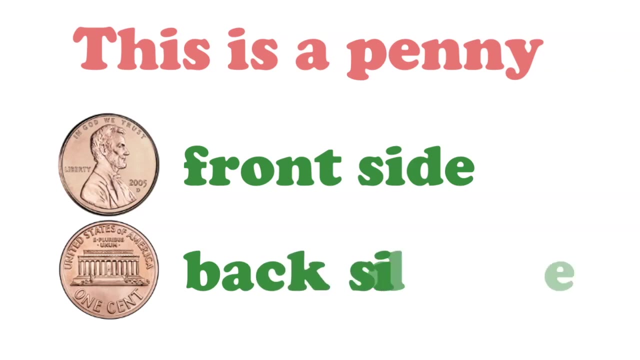 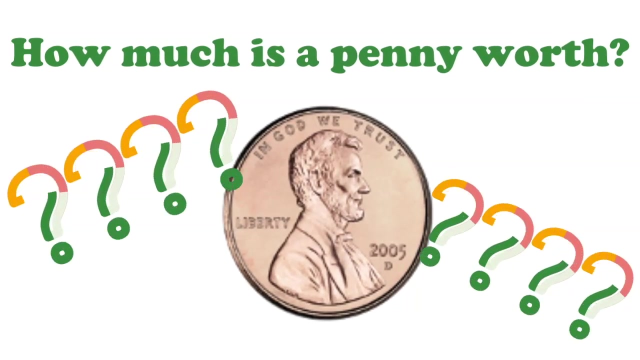 100.. 5, 100, 20 nickels equals 100 cents. 100 cents equals 1 dollar. This is a penny. This is the front side and this is the back side. How much does a penny work, Do you know? 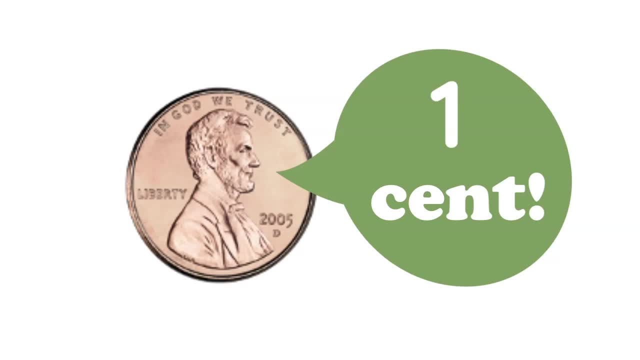 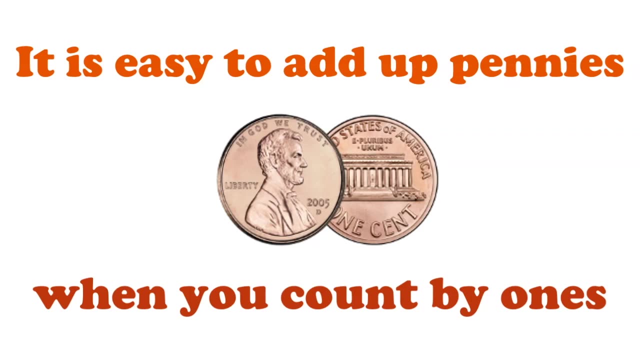 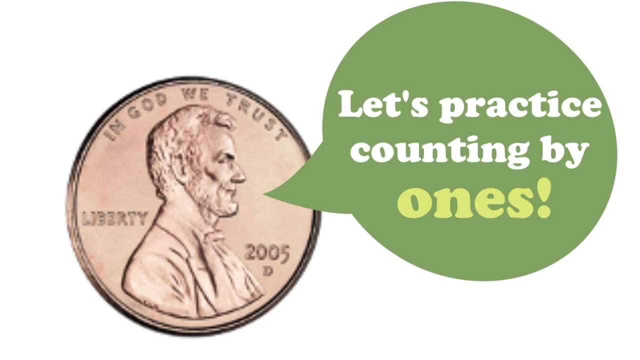 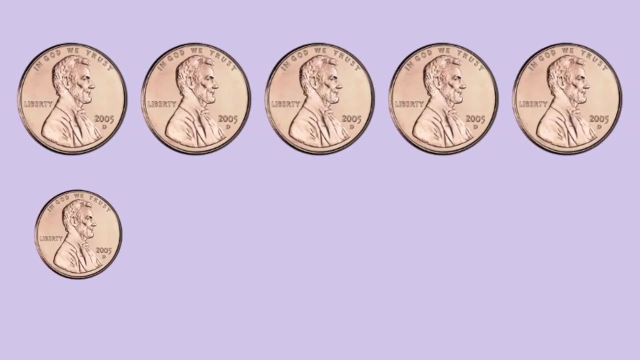 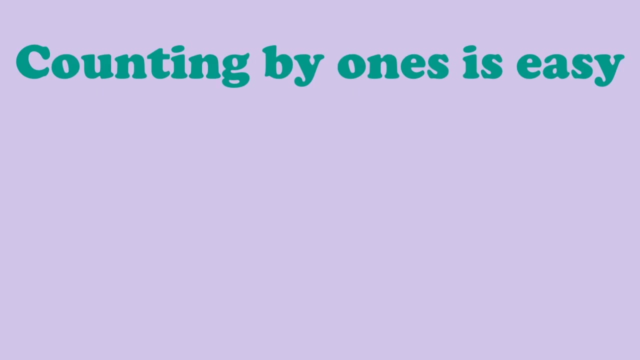 Yes, it is worth one cent. It is easy to add up pennies when you count by ones. Let's practice counting by ones: One, two, three, four, five, six, seven, eight, nine, ten. Counting by ones is easy, but grouping by tens is easier. 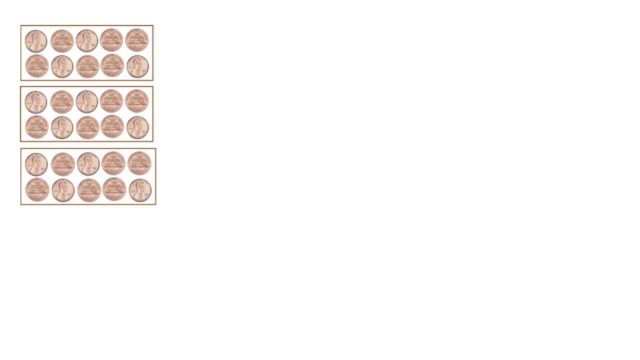 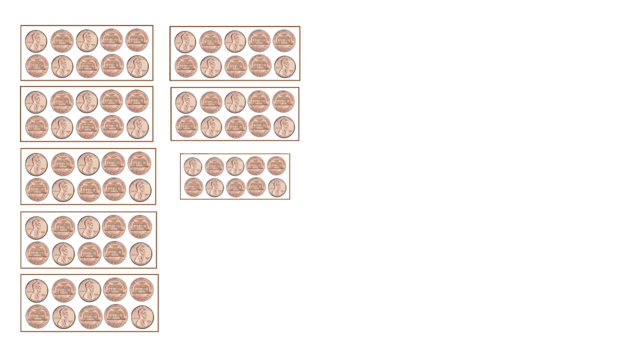 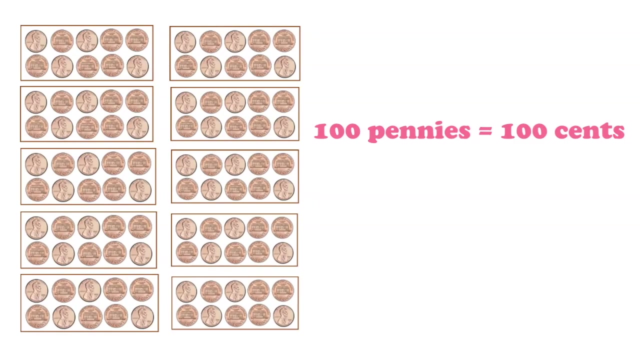 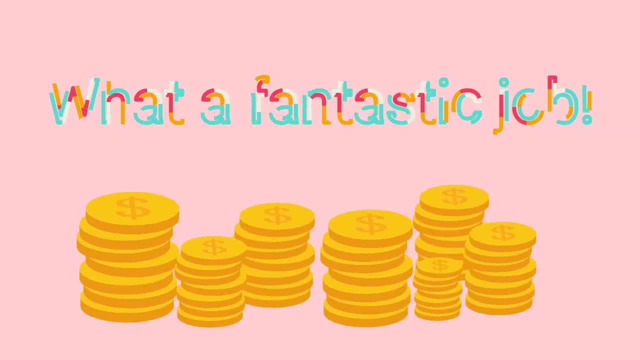 Ten, twenty, thirty, forty, fifty, sixty, seventy, eighty, ninety, one hundred One hundred pennies equals one hundred cents. One hundred cents equals one hundred cents One dollar. What a fantastic job. You are now an expert. 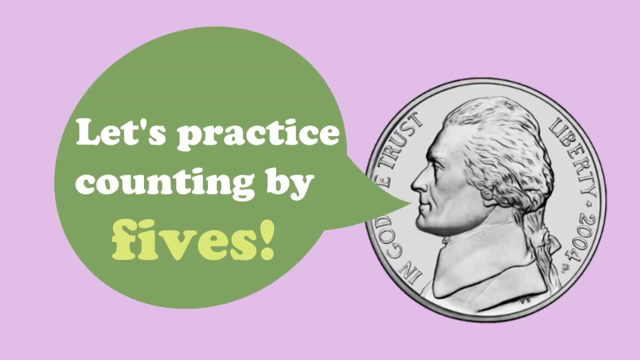 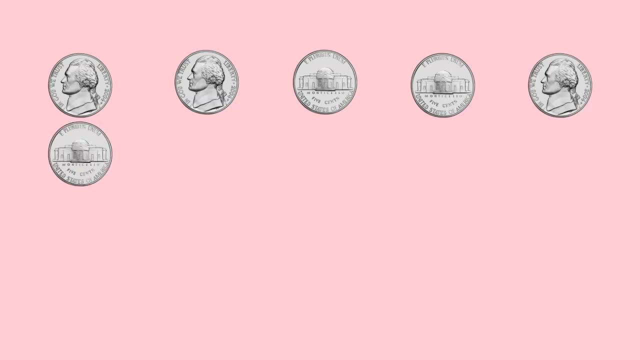 Let's practice counting by fives: 5,, 10,, 15,, 20,, 25,, 30,, 35,, 40,, 45,, 50,, 55,, 60,, 65,, 70,, 75,, 80,, 85,, 90,, 95,, 60,, 75,, 80,. 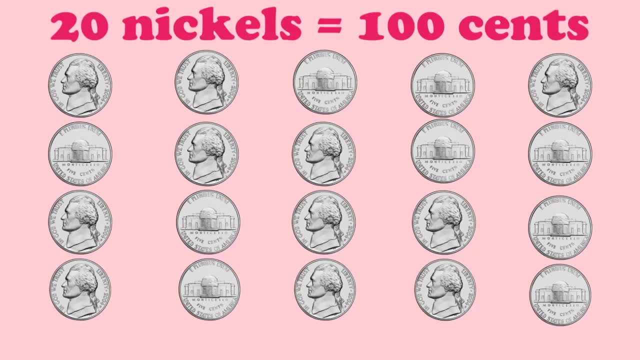 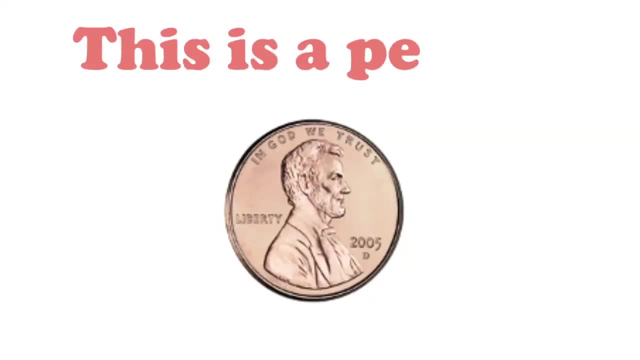 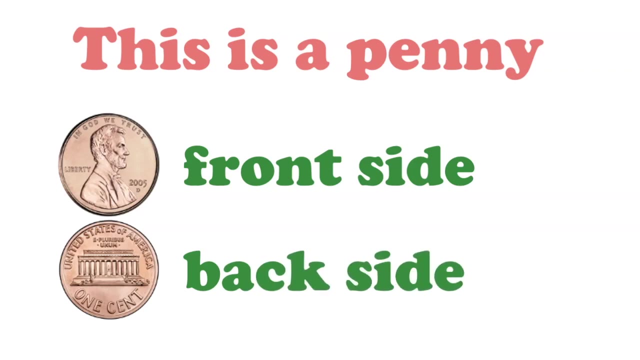 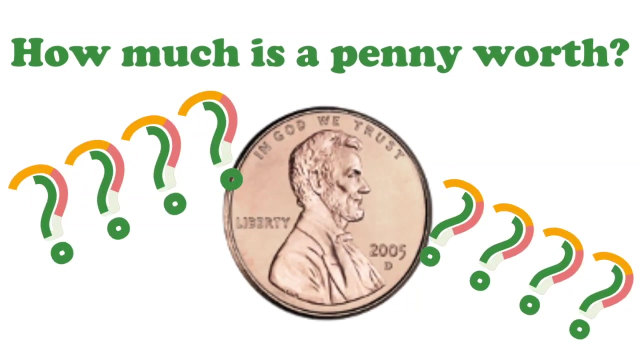 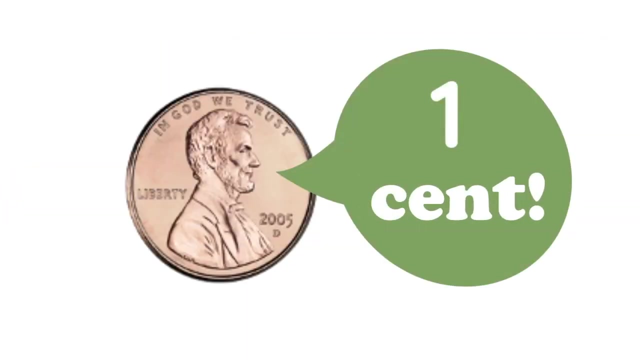 100.. 20 nickels equals 100 cents. 100 cents equals 1 dollar. This is a penny. This is the front side and this is the back side. How much is a penny worth, Do you know? Yes, it is worth 1 cent. 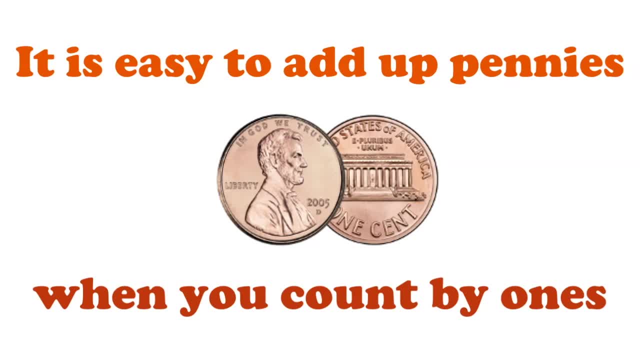 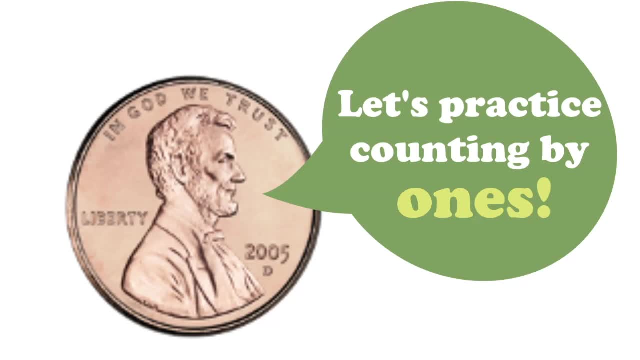 It is easy to add up pennies when you count by ones. Let's practice counting by ones: 1, 2,, 3,, 4,, 5,, 6,, 7,, 8,, 9,, 10.. 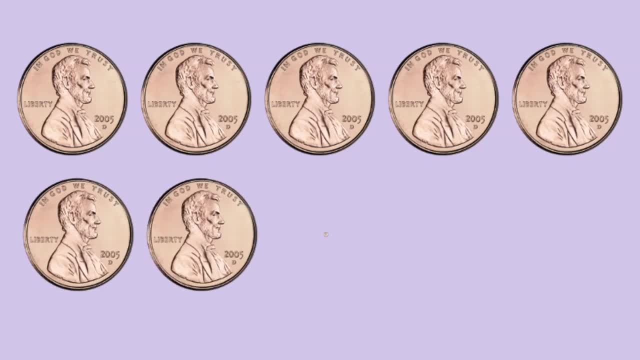 1,, 2,, 3,, 4,, 5,, 6,, 7,, 8,, 9, 10.. 1, 2,, 3,, 4,, 5,, 6,, 7,, 8,, 9, 10.. 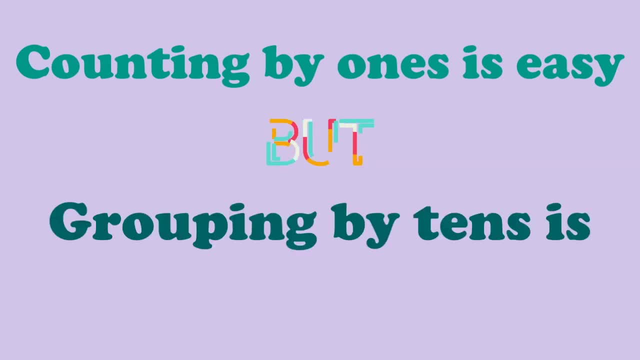 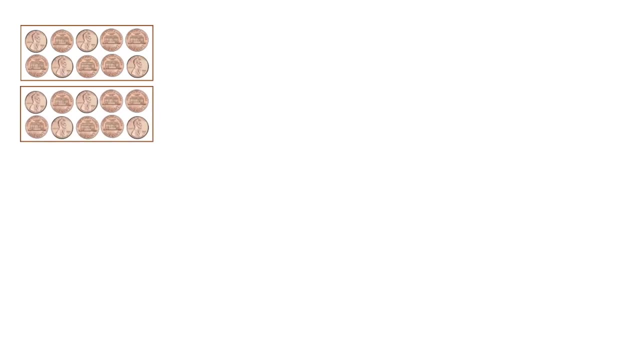 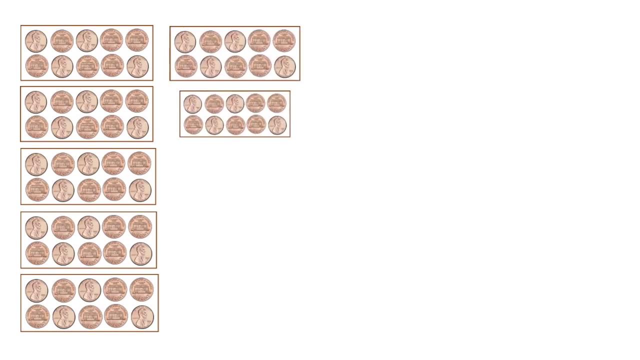 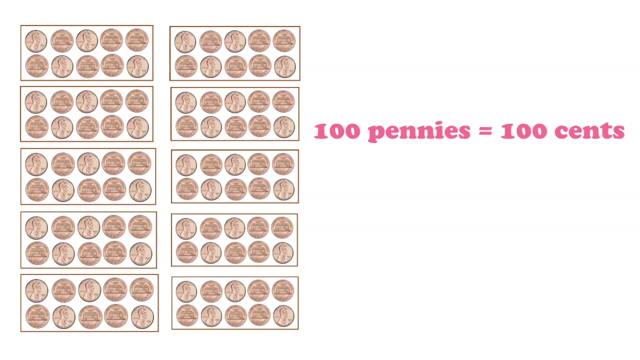 Counting by ones is easy, but grouping by tens is easier: 10,, 20,, 30,, 40,, 50,, 60,, 70,, 80,, 90, 100.. 100 pennies equals 100 cents. 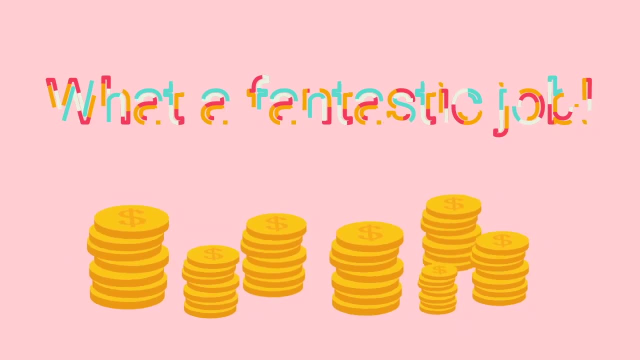 100 cents equals 1 dollar. What a fantastic job. You are now an expert.